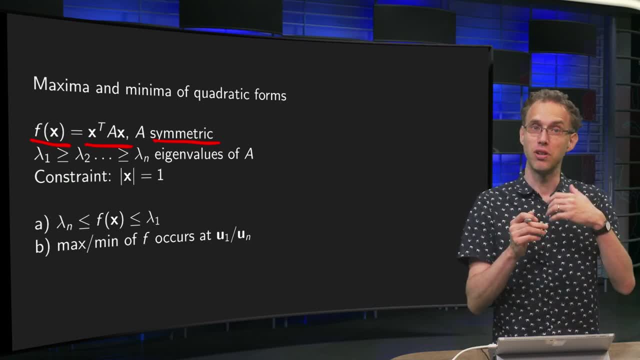 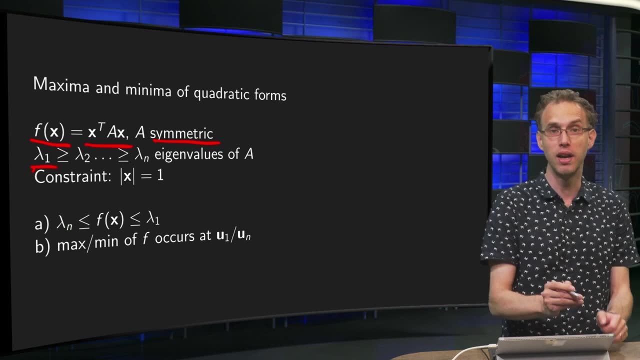 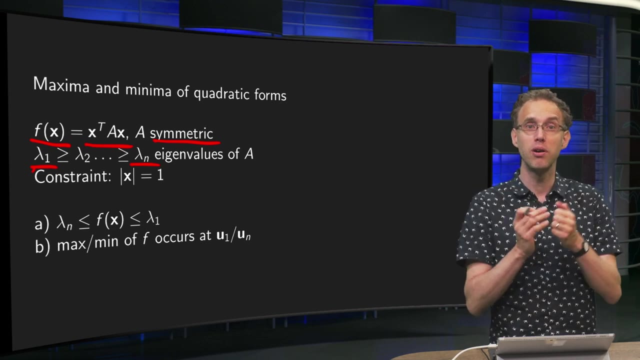 so we know that all eigenvalues are real. so we have lambda 1 up to lambda n real eigenvalues and let's put them with the biggest first. So lambda 1, biggest eigenvalue, until lambda n, the smallest eigenvalue. Now we are going to find an optimum of this function with a constraint. 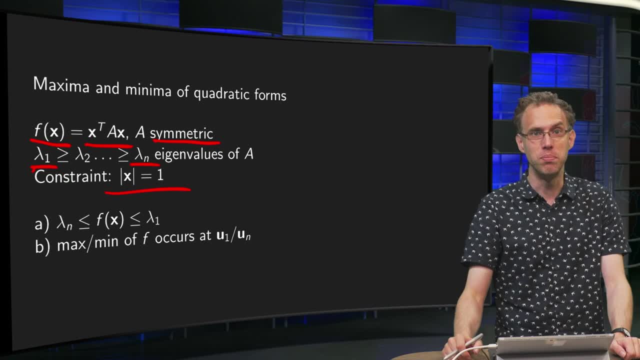 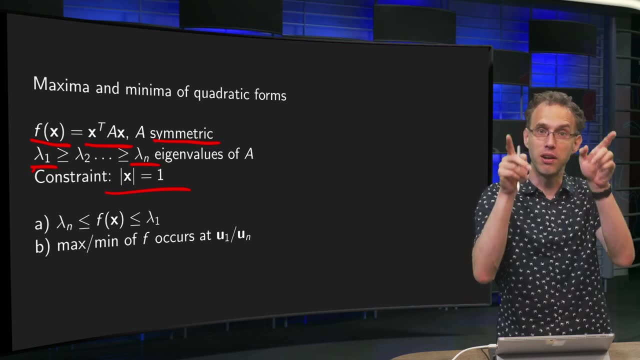 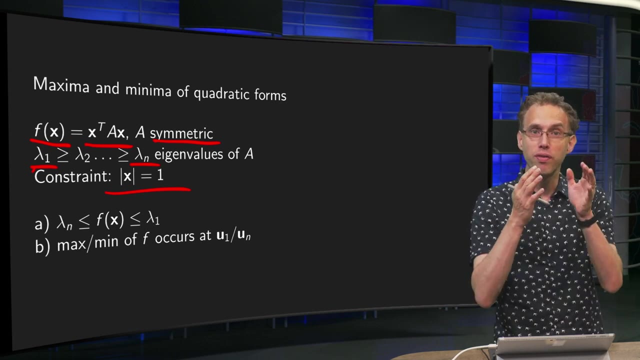 The input variable in norm has to be 1.. So what does that mean? If your x is in R2, for example, norm is 1, means that we are looking for a point lying on the circle. x1 squared plus x2 squared equals 1, and we are trying to find the optimum of our 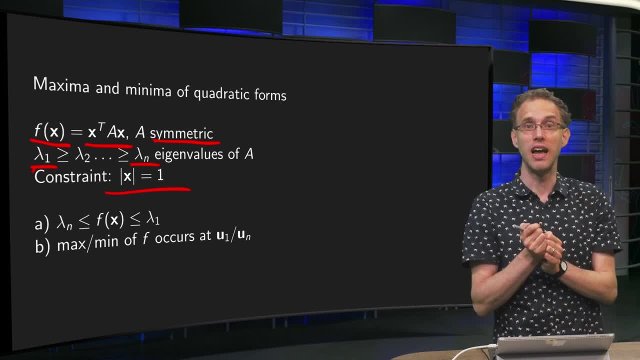 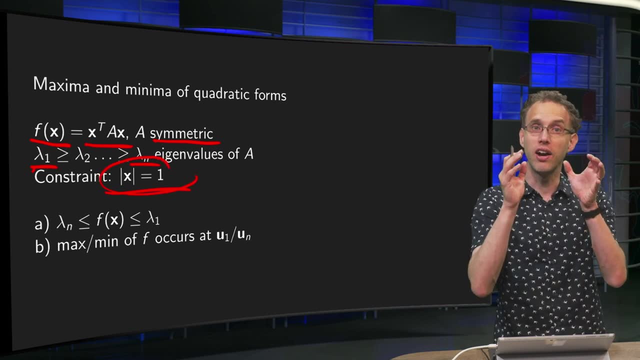 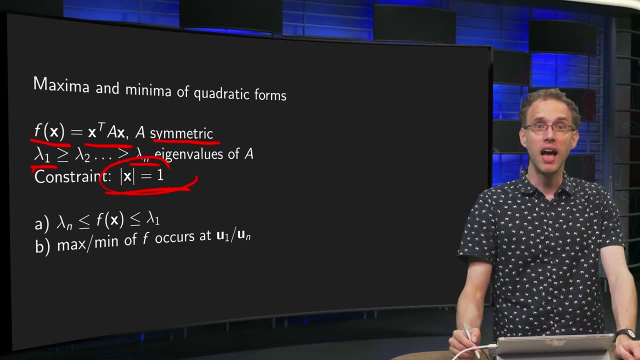 f under the constraint that our input variable lies on a circle, Or if x is in R3, then this constraint means that our input variable lies on a sphere. So with that constraint we are trying to optimize our function f. Now, usually if you have some general function f, you can do this. 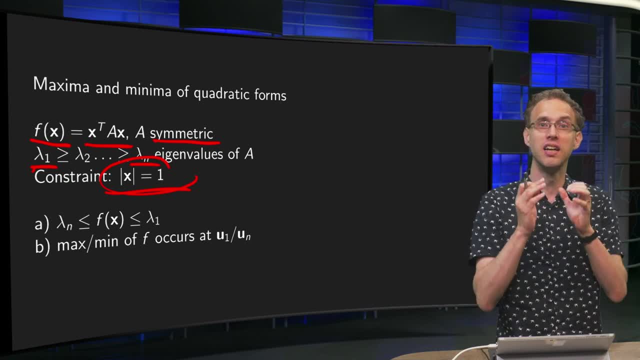 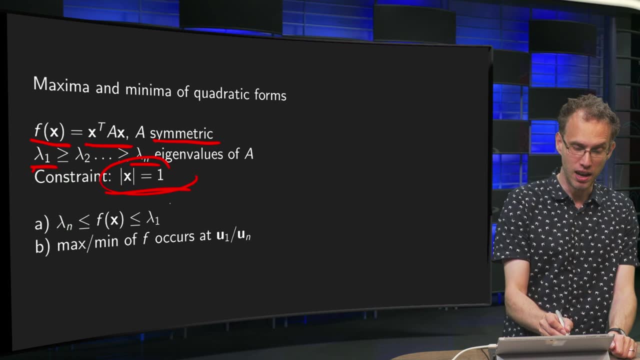 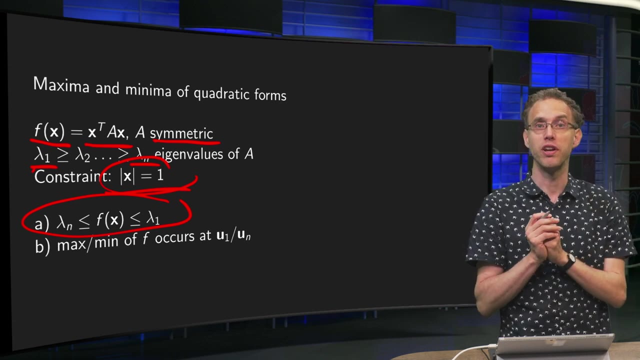 then you need Lagrange multipliers and you get a lot of computations. However, in this case it is a lot easier because we have a theorem that says that our f lies in between the biggest and smallest eigenvalue, So f is always smaller than the. 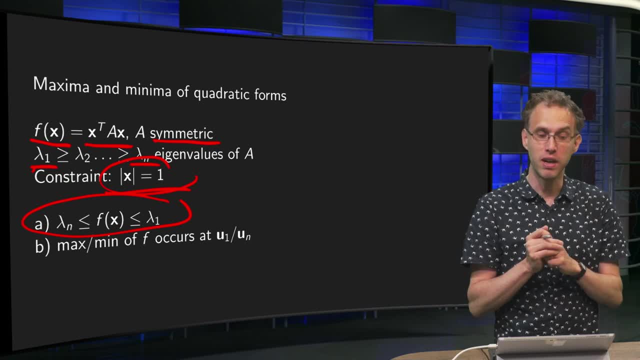 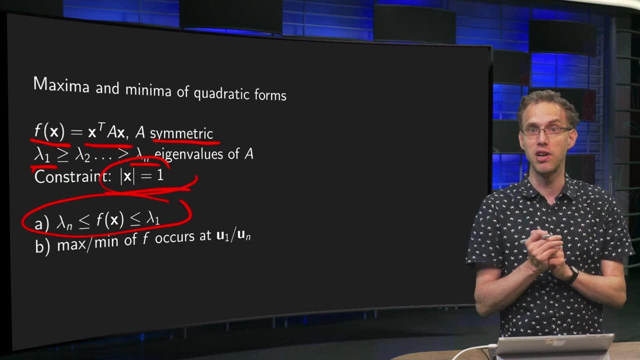 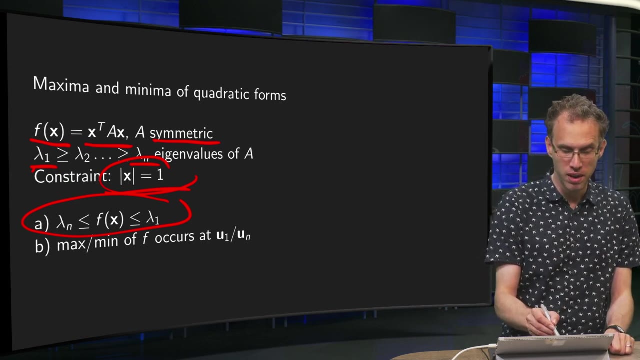 biggest eigenvalue and f is everywhere bigger than the smallest one. And it also tells you where you can find this optimum. So the maximum is lambda n and the minimum is lambda 1.. And the theorem also tells you where you can find it And the maximum occurs at the. 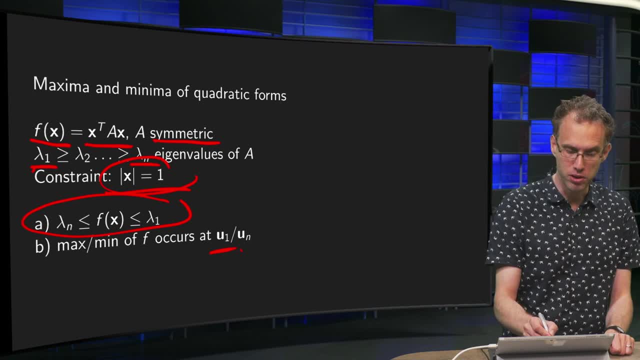 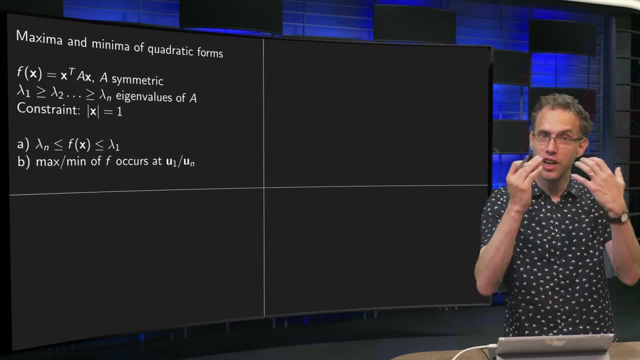 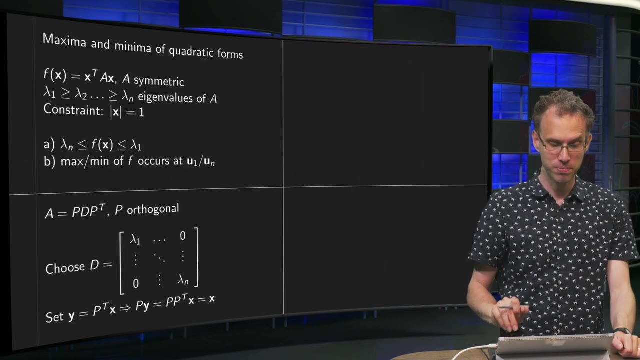 biggest eigenvalue, So at u1.. And the minimum occurs at the smallest eigenvalue, at un. So we already know straight away where our maximum and where our minimum is, what the maximum is and what the minimum is. Well, why is that? Well, we have a symmetric matrix A, So let's prove this. 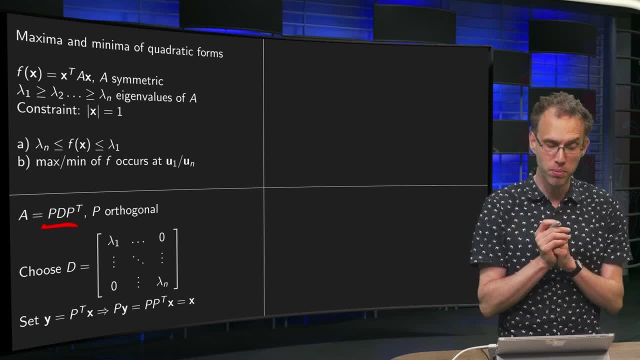 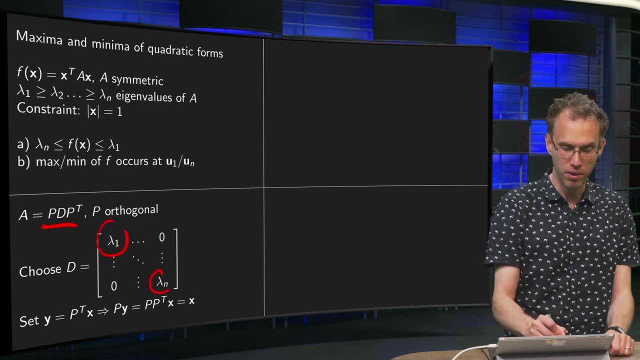 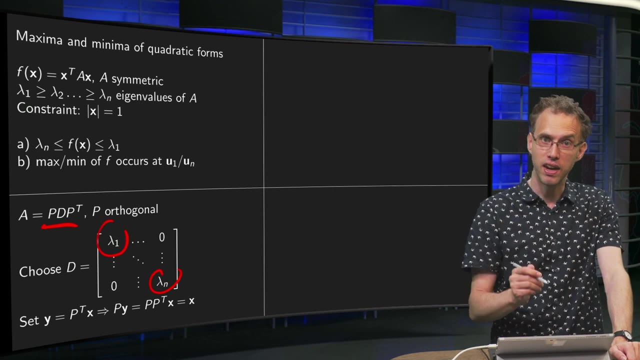 A is a PD, P transpose, where P is an orthogonal matrix. And we construct it such that we put our lambda 1 over here and our lambda n over there. So we start with the biggest eigenvalue and with the smallest eigenvalue And then we define a new variable: y, y equals P transpose times x. 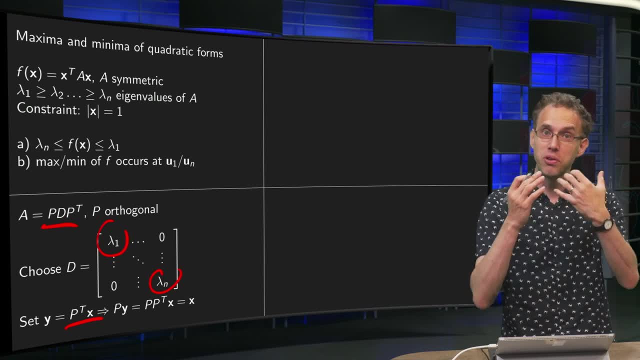 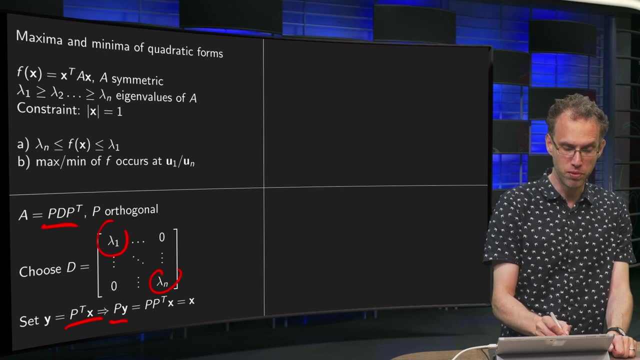 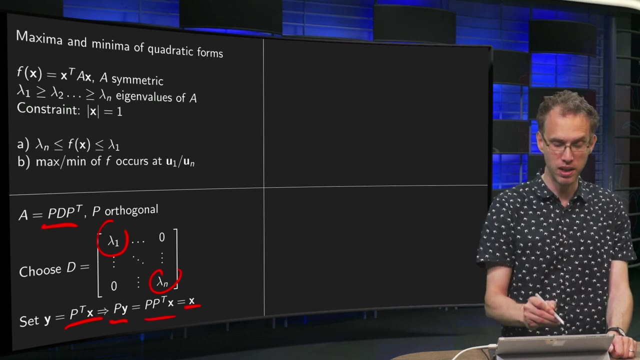 because in this new variable y, our function, our quadratic form becomes a lot easier. Why is that? Well, multiply by P, then you see: P times y equals P, P transpose x. but P times P transpose is identity matrix, Because P is orthogonal, so we get x, So we have both: y equals P transpose times x and P times y. 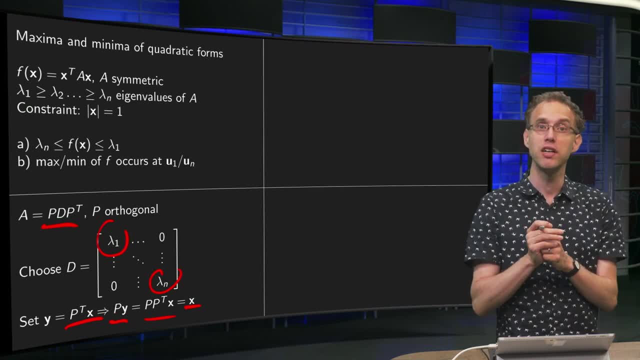 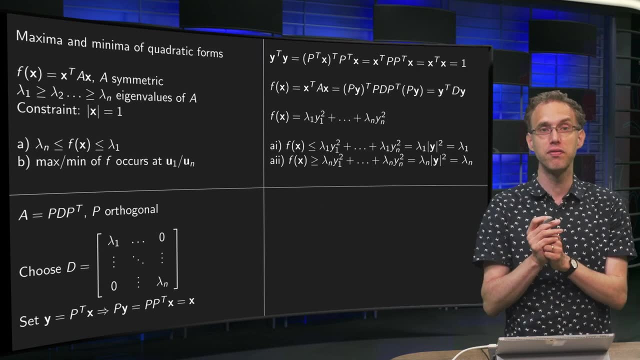 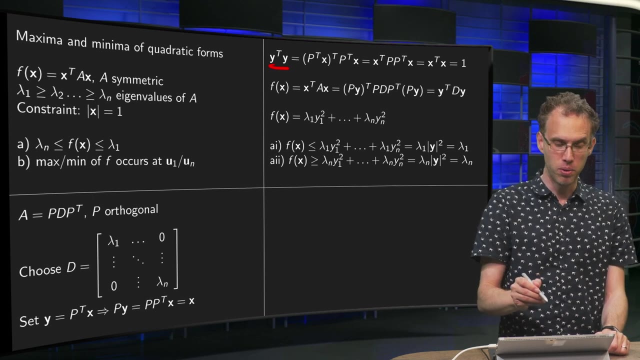 equals x. Now our x is normalized. We will show first that our y is normalized as well. So we compute the inner product of y with itself, And this is the same as computing y transpose times y. So that's what we do over here. We know that y equals P transpose times x. So we have the 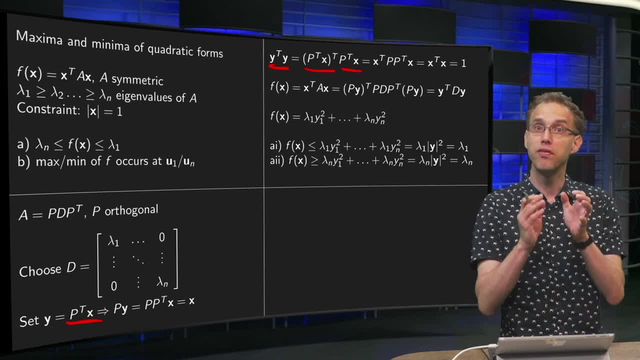 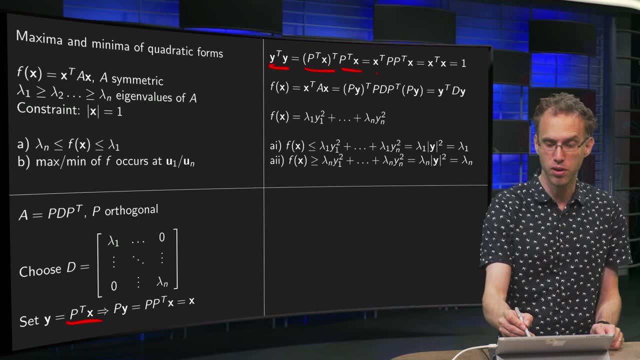 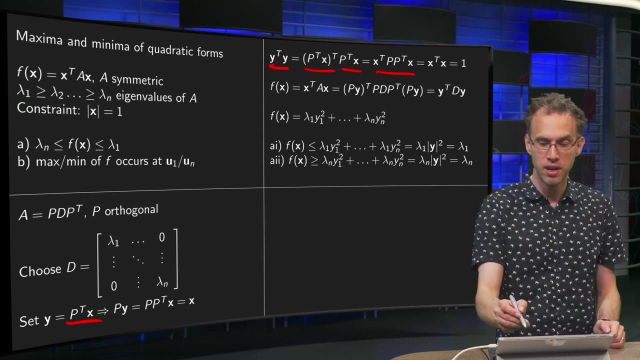 y transpose times y. Now, if you take the transpose of a product, you take the product of the transposes in opposite order. So that's what we do over here. So we get x transpose times P transpose transpose, which is P times P transpose times x. However, 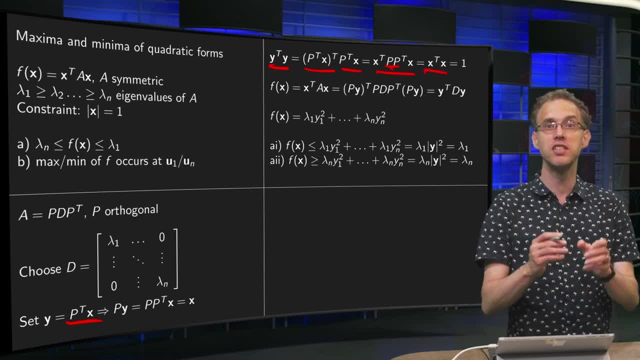 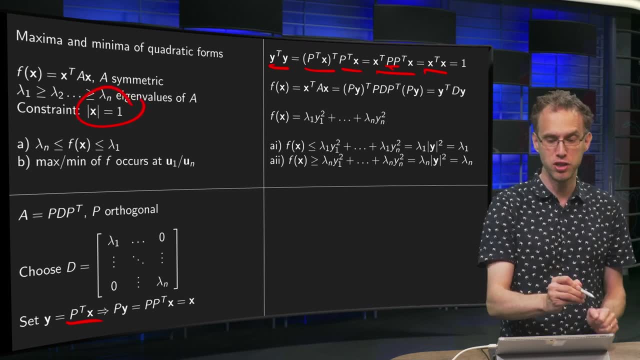 this term. in the middle is again identity. So we get x transpose times x, But x transpose times x is the same as x inner product with x, but x was normalized. So this is 1.. So it means that the 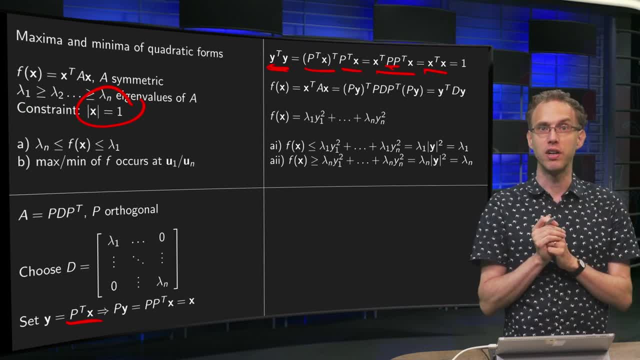 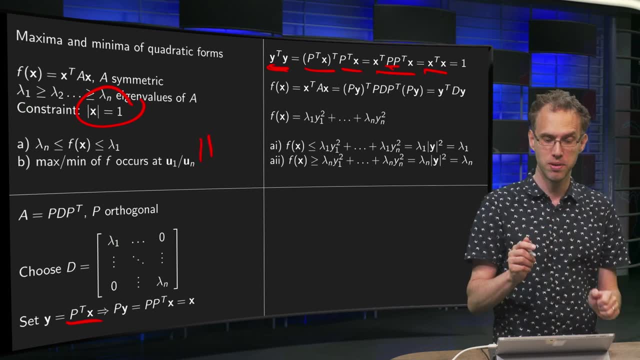 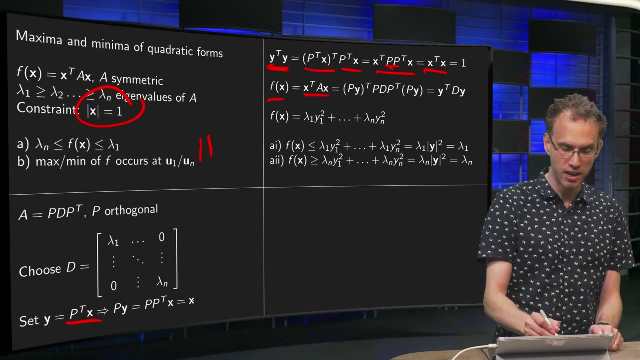 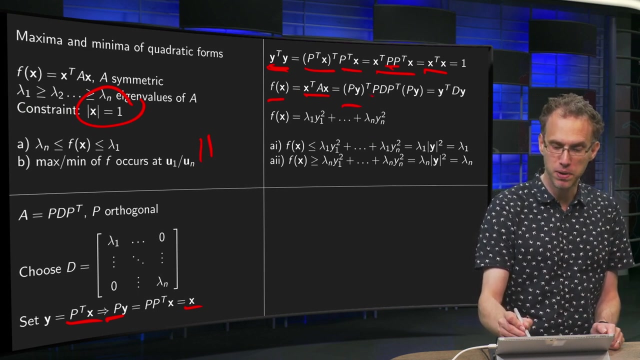 y is also normalized. Okay, so a lot of work has been done. Now we can show what we want to show as follows. So we know that our f of x equals x transpose times A times x. Now we replace the x by P times y. So here we have x transpose And we replace A by P transpose. 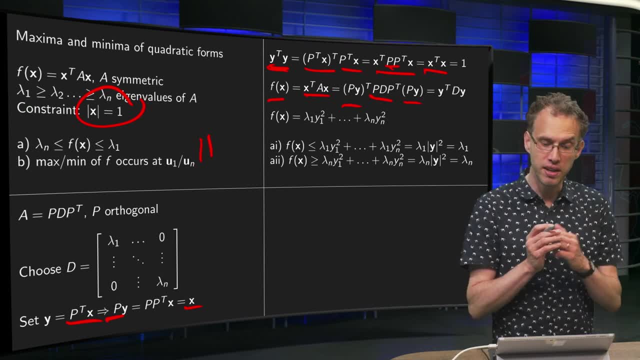 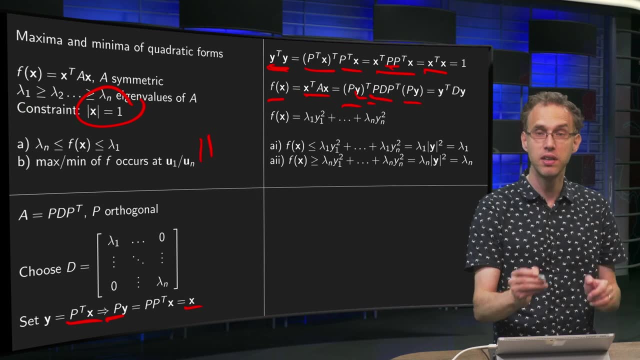 And we replace the x again by P times y And Then we get: if you work out the product, we get y. transpose times p. transpose times p. cancels out times d. times p. transpose times p. again identity times y. 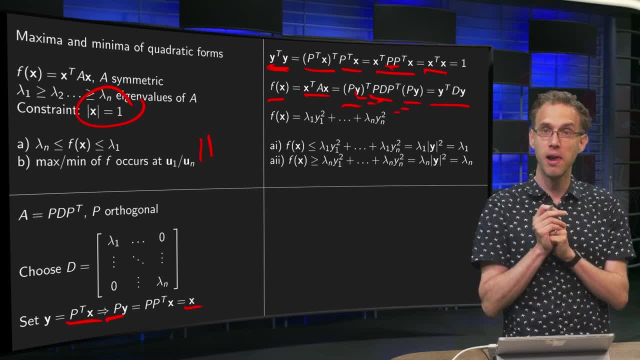 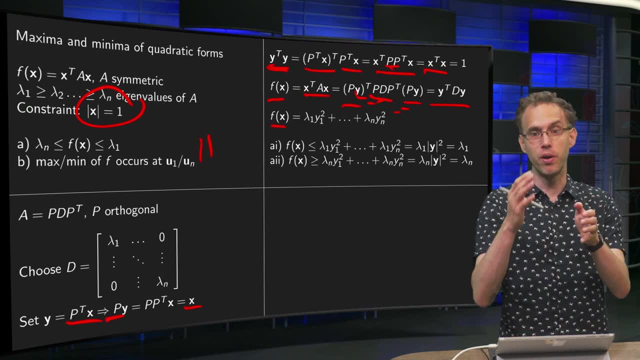 So we are just left with y transpose times d times y. So if we express our f in terms of our new variable y, we just get f of x equals lambda 1 y1 squared, plus lambda 2 y2 squared, and so on, plus lambda n times y n squared. 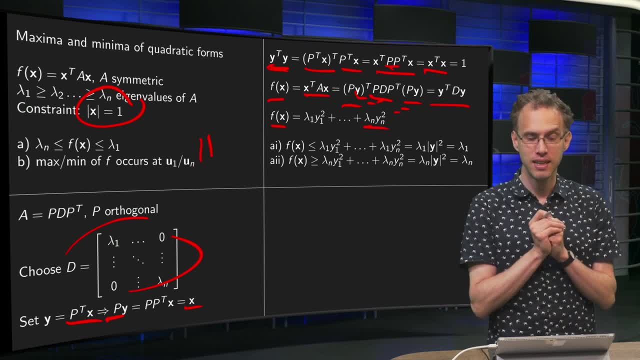 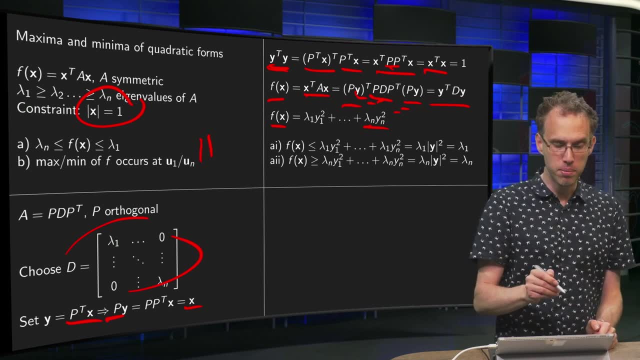 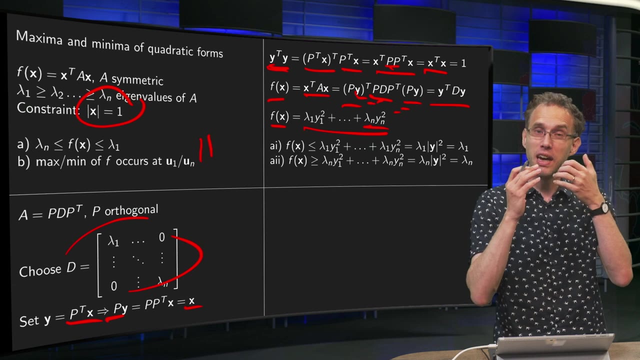 Because we just have a diagonal matrix in between, And that's nice because now we can use the following trick: Now the lambda 1 is the biggest eigenvalue. So if you replace all lambda's over here by lambda 1, we make this expression on the right-hand side bigger. 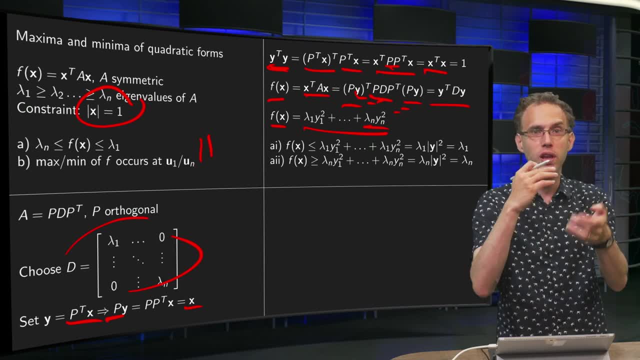 Because all the y1 squared are positive. so if we are going to replace all lambda's, we turn them all in lambda 1, then we make all terms bigger. So we have a diagonal matrix in between. So if we replace all lambda's over here by lambda 1, then we make all terms bigger. 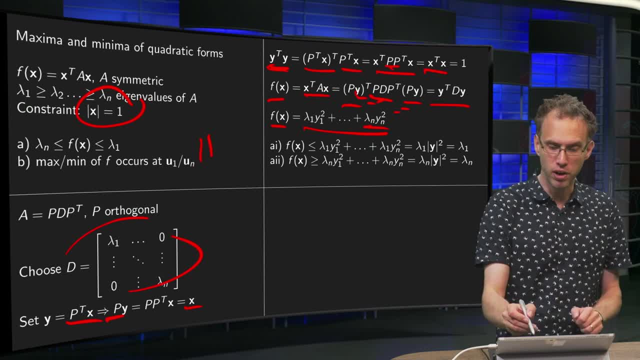 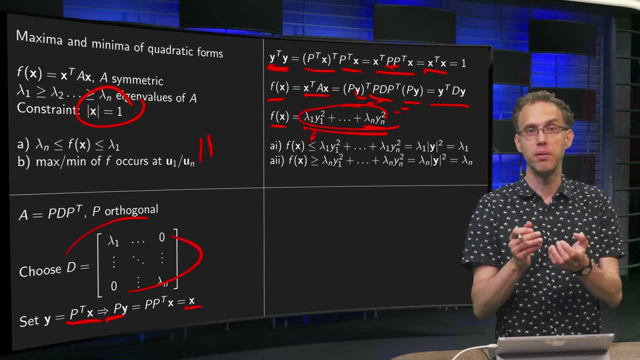 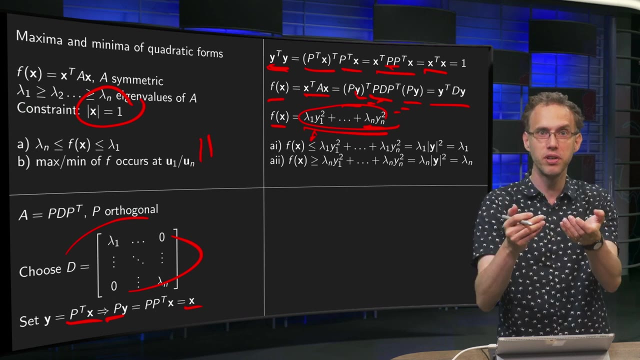 So that means that the f is in fact smaller than this expression over here, where all lambda's have been replaced by lambda 1.. That's what we do over there Now, and then we are basically done. We take the lambda 1 out and we get lambda 1 times y1 squared plus y2 squared plus y3 squared, and so on. 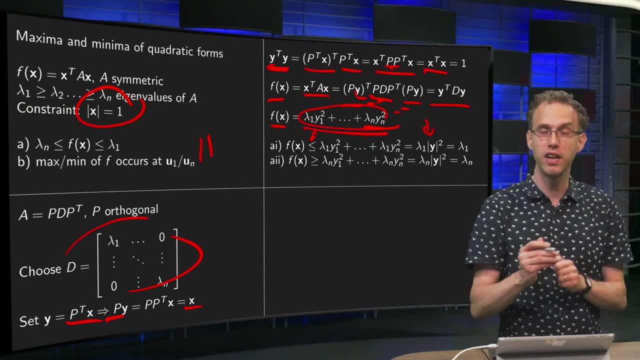 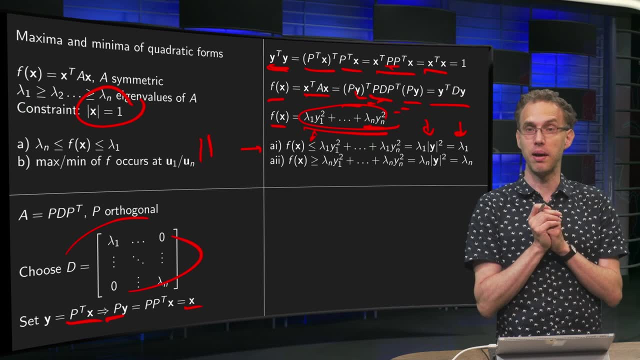 So that's lambda 1 times the normal phi squared. That's what we have over here, But the normal phi squared equals 1, so we end up with lambda 1.. So there we have that f is smaller or equal than lambda n. 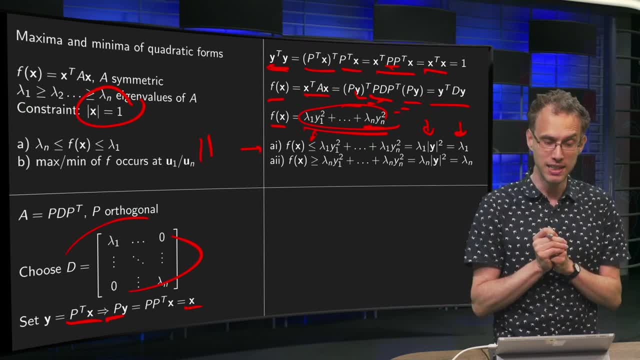 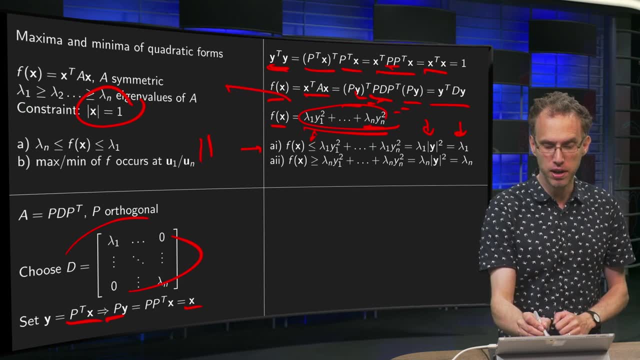 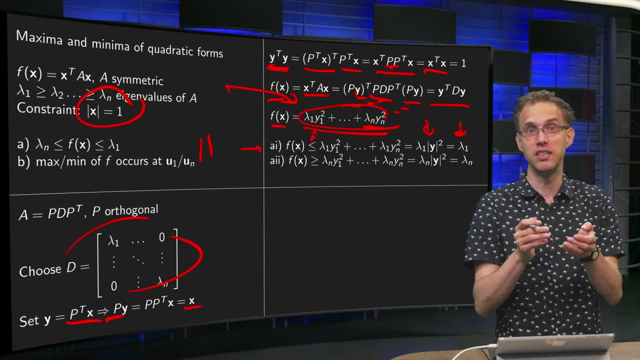 Now we can do a similar trick with the lambda n's. So the lambda n is the smallest eigenvalue. So if we replace all eigenvalues in this right-hand side by a lambda n, we make the whole expression smaller, which means that the function f is bigger than this expression. if we put lambda n's everywhere, 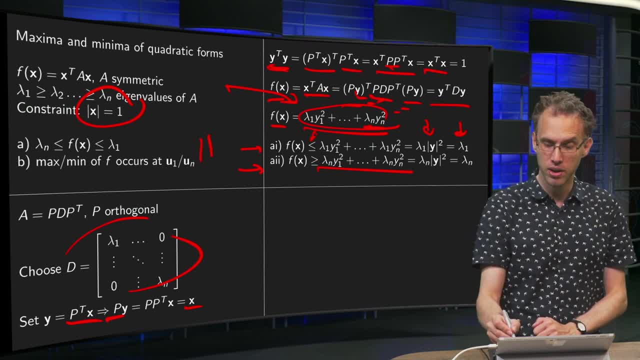 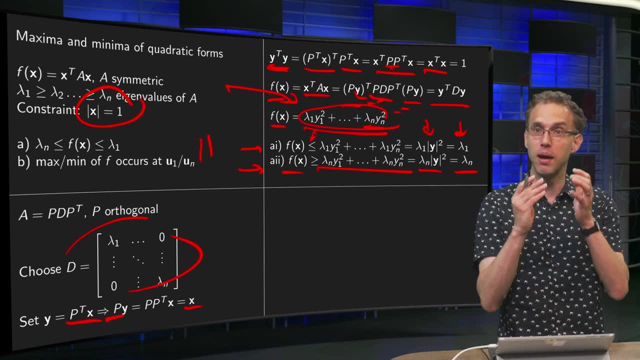 And then we have the same argument. You can take the lambda n out, You get lambda n times 2. That's the normal phi squared, which is just lambda n. So f is bigger or equal than lambda n everywhere. And then we have proven the first part. 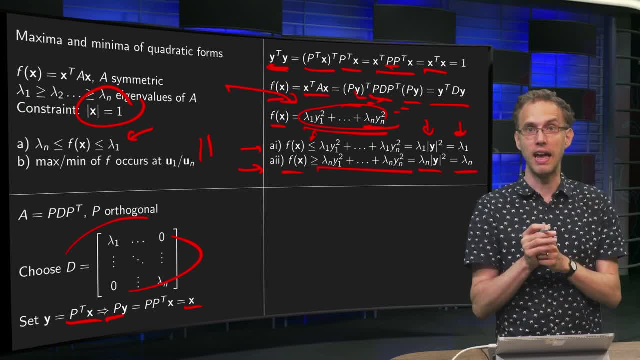 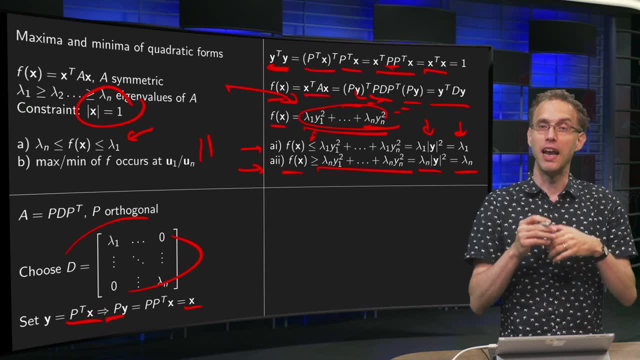 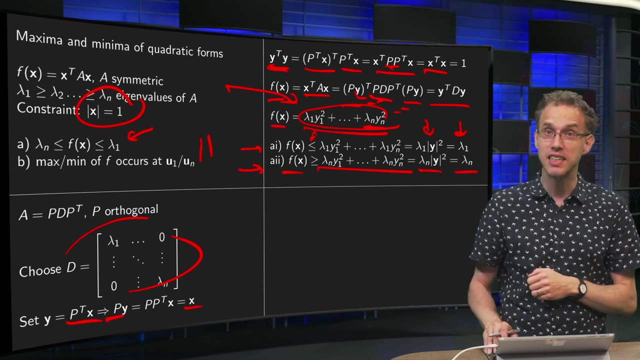 So f is smaller than lambda 1, and f is bigger than lambda n. So the maximum, if it occurs, is the function at most lambda 1, and a minimal value. you cannot go below lambda n. So do we actually attain these points? 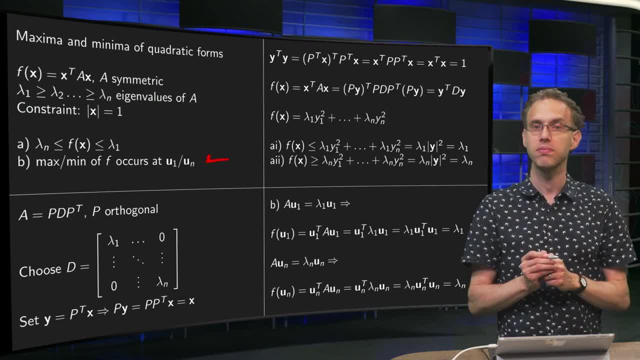 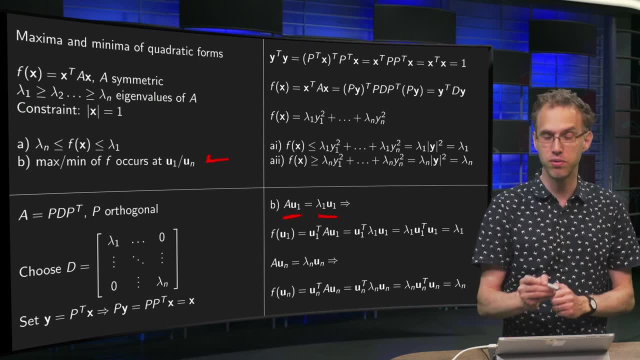 Well, yes, we do. That is the second part. We take a normalized eigenvector u1 belonging to lambda 1.. So we have a times u1 equals lambda 1 times u1.. Plug it into your f, your f of u1. 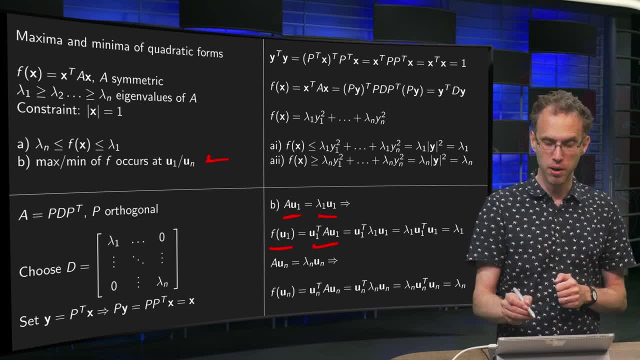 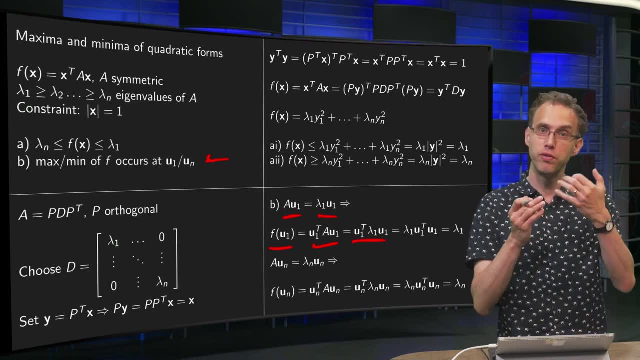 So what do you get? u1 transpose au1.. But a times u1 equals lambda 1 times u1.. Take the lambda 1 out. You get u1 transpose times u1.. But we took a normalized eigenvector. 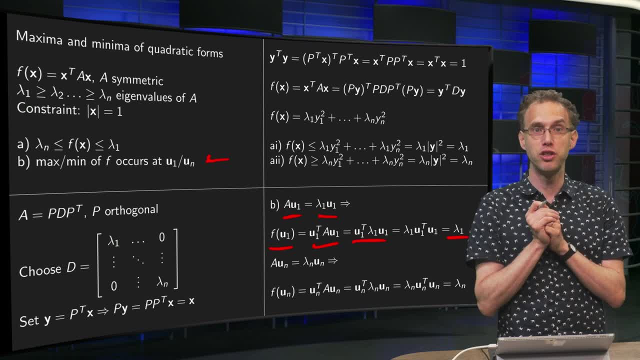 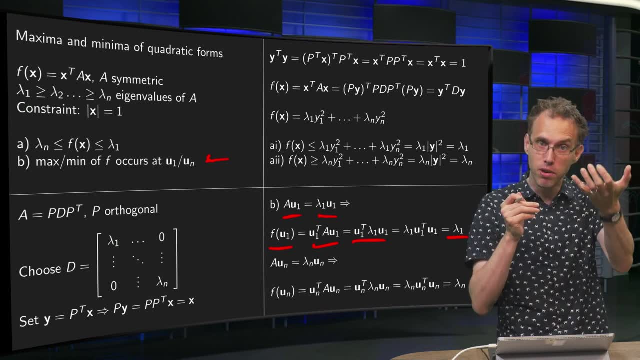 So that's 1.. So we get lambda 1. So the f at u1 equals lambda 1. So that's the maximum value. You can be at most lambda 1. You reach that value at u1.. 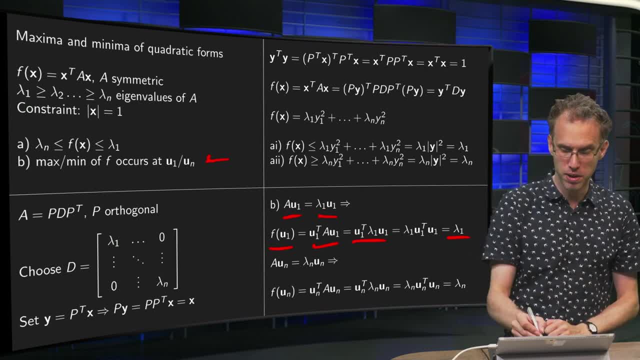 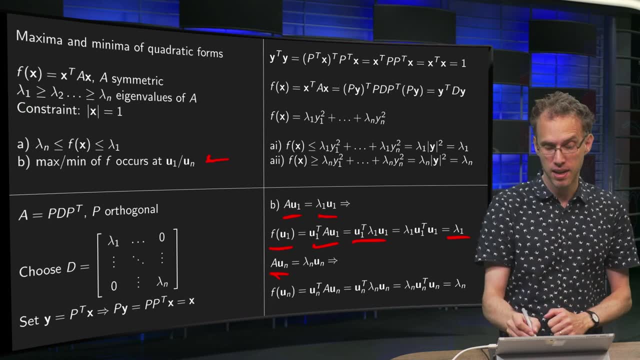 So that's your maximum, And similarly for the minimum. then you take u and the eigenvector, normalized eigenvector belonging to lambda n. You know a times u and equals lambda n times u, and plug it in And the f at u1 is then u1. transpose au1.. 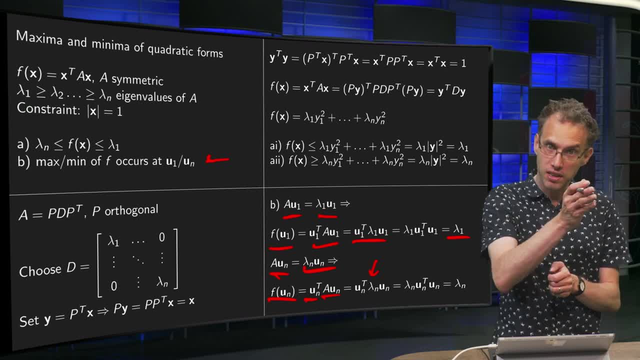 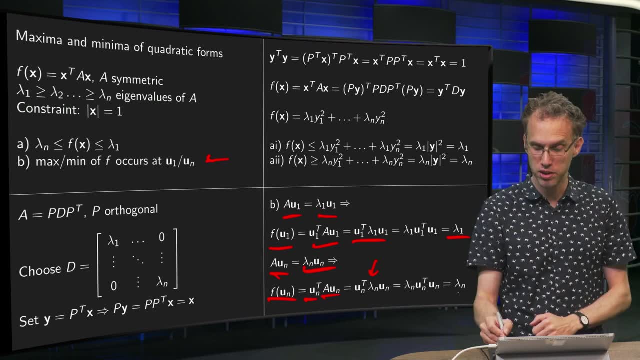 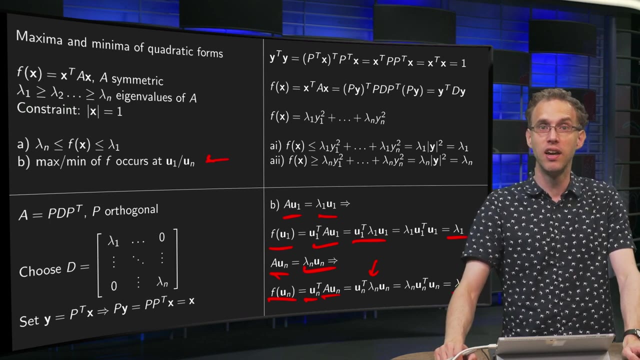 A times u1 equals lambda n times u1.. Take the lambda n in front. You get u1. transpose u1.. That's the norm of u1. But the eigenvector was normalized, So you get lambda n. So we also attain the minimum at u1 and its value is lambda n. 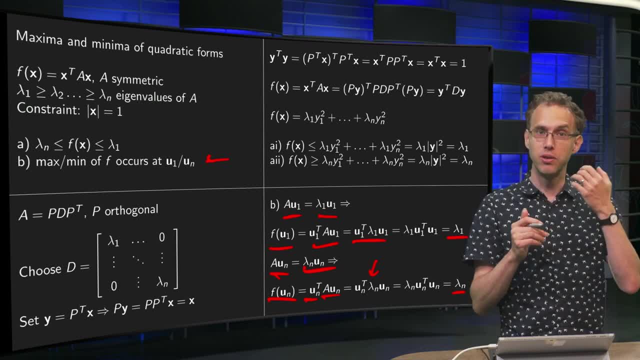 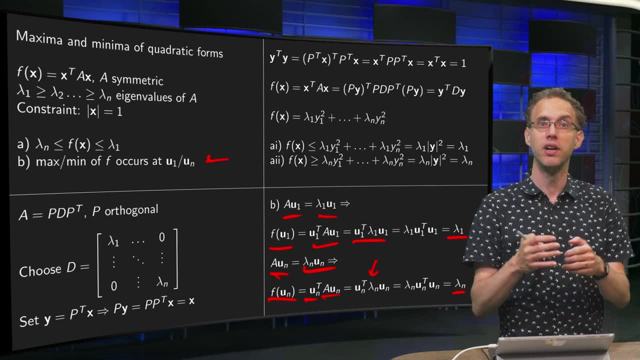 So there we are. If you have a quadratic form, you know what the maximum is- The biggest eigenvalue- You know what the minimum is- Smallest eigenvalue- And you know that you will attain them and where you will attain them. Thank you. 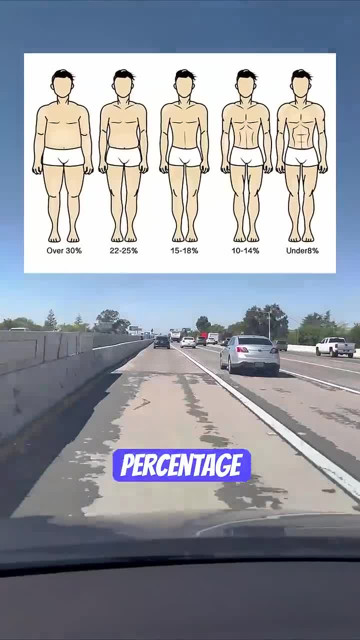 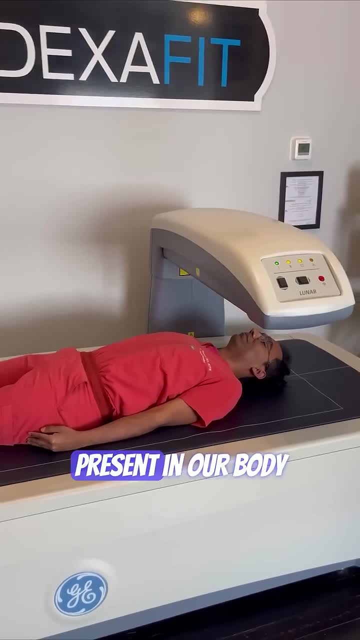 I decided to get a DEXA scan to assess my body fat percentage because I belong to the category called skinny fat. DEXA is a body scan which accurately estimates how much fat is present in our body, though you don't look overweight, So you're in the above average area. The goal. 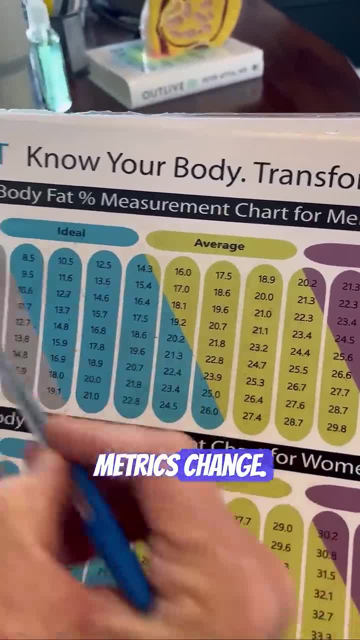 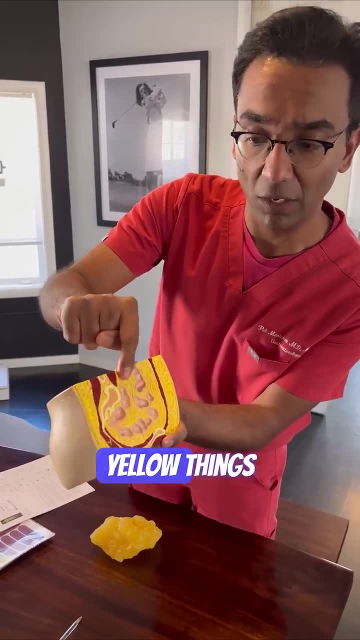 would be initially to get you here into the average where the health metrics change. So for you that would be getting to 20 percent. 20 plus is over here. So, guys, this little fat I'm talking about, look at this. these are the yellow things that are surrounding your organs inside your